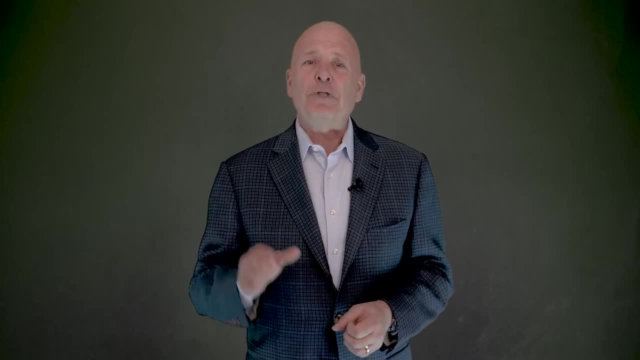 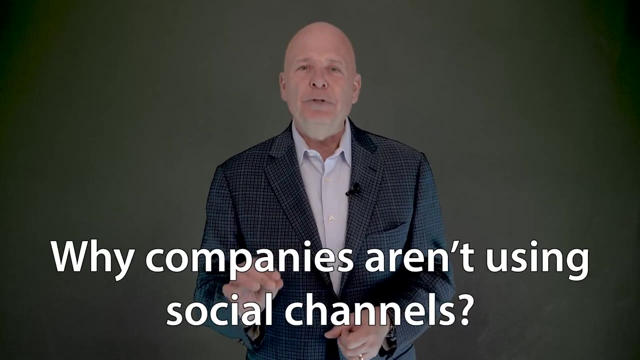 that doesn't mean it's not important. More and more customers turn to social media to get help. More on why in just a moment, but for now let's address why companies aren't using social channels. When a company tells me they don't want to participate in social 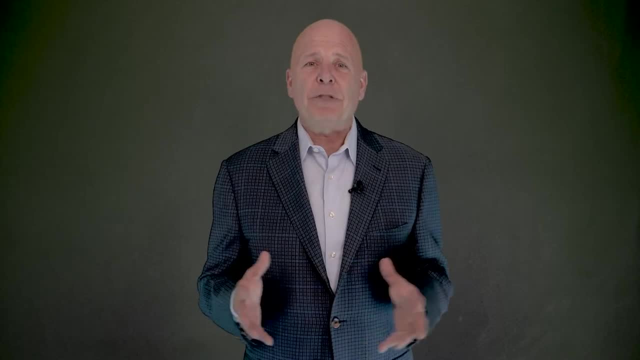 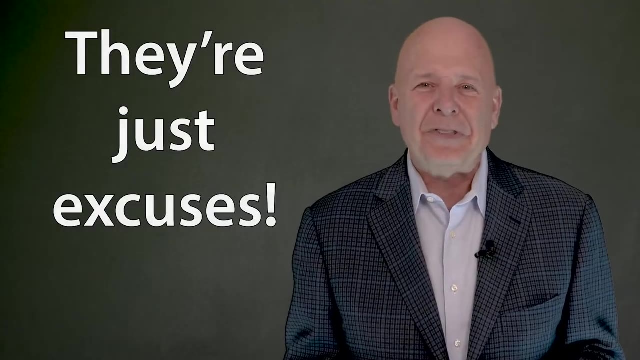 media customer care. I ask why? and they have all kinds of explanations. Now notice I'm avoiding the word excuses, but that's exactly what they are. They're just excuses. So the explanations they share are number one. we steer them to the phone, so we don't need any. 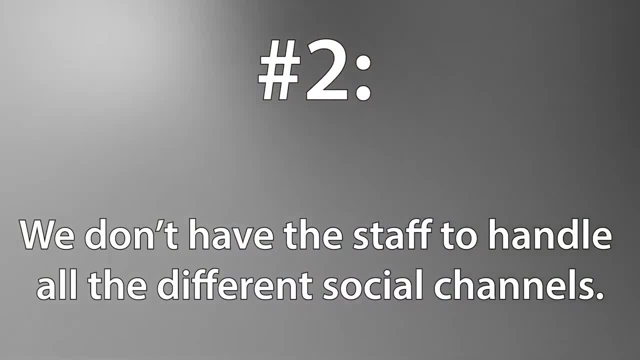 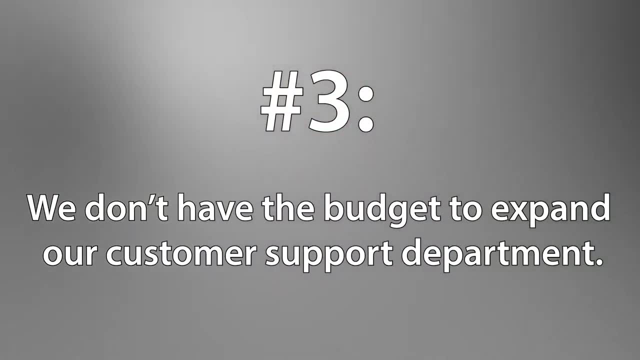 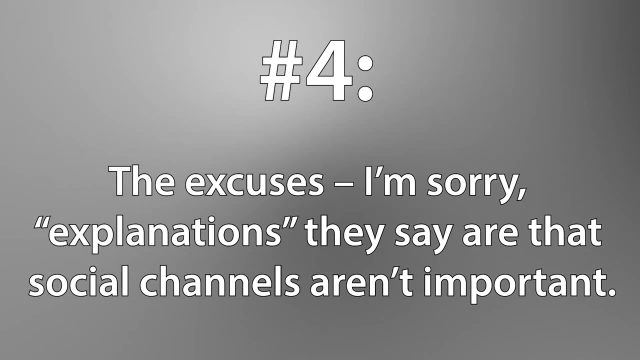 other channels. Number two: We don't have the staff to handle all the different social channels. Number three, we don't have the budget to expand our customer support department. And number four, the excuses, I'm sorry, explanations. The explanations, they say, are that social channels aren't important. 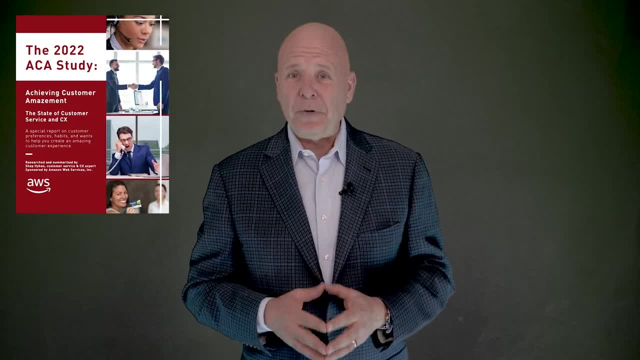 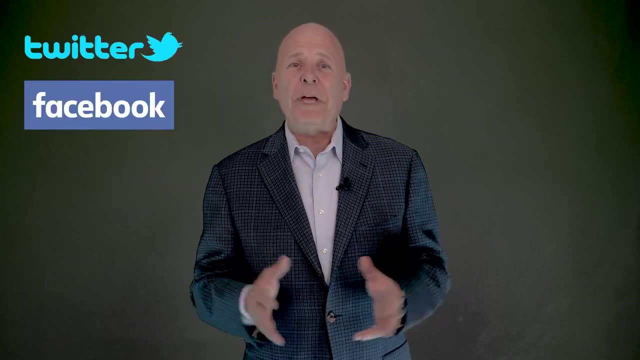 Well, our annual customer service research shows that, of all the ways customers reach out to customer support, social media channels like Twitter, Facebook, Instagram, Twitter, Facebook, Instagram and others are at the bottom of the list. but that doesn't mean. 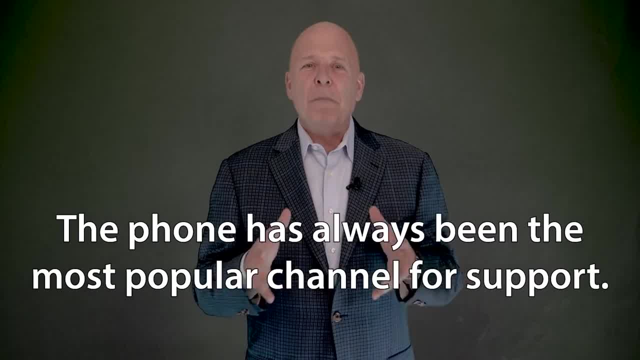 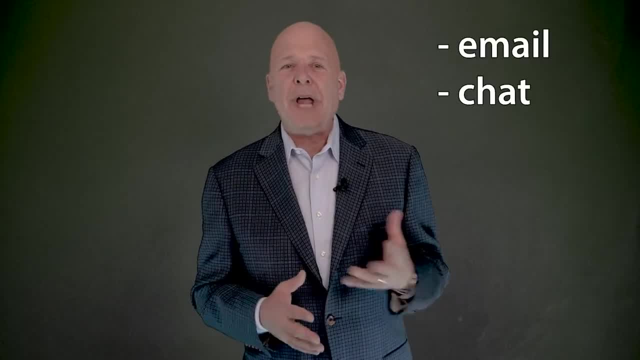 they should be ignored. The phone has always been the most popular channel. Why? Well, because it's easy and it's always been there. but now there are options such as email, chat apps and more Well, Gen Z and millennials are the catalyst of digital customer support. 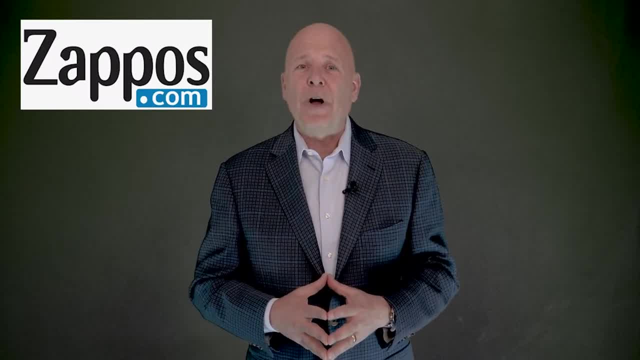 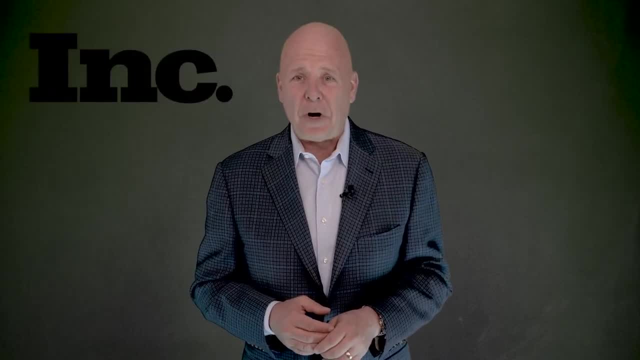 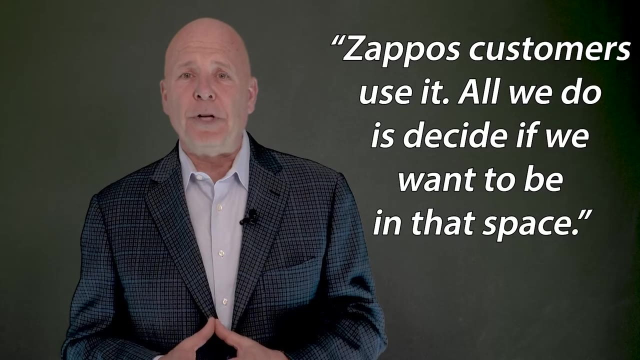 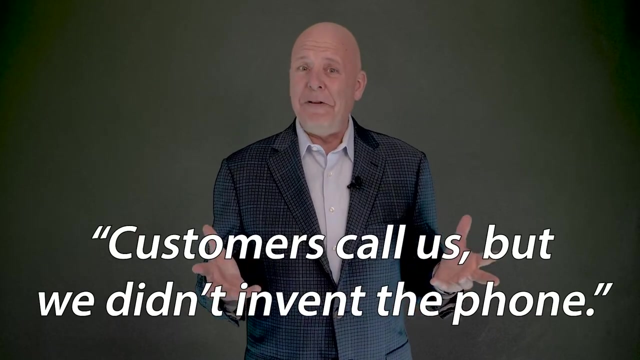 channels. Zapposcom's former senior director of customer loyalty, Bob Seifker, shared his take on social media. Zappos uses social media. His answer was: Zappos customers use it. All we do is decide if we want to be in that space. He also said: customers call us, but we didn't invent the. 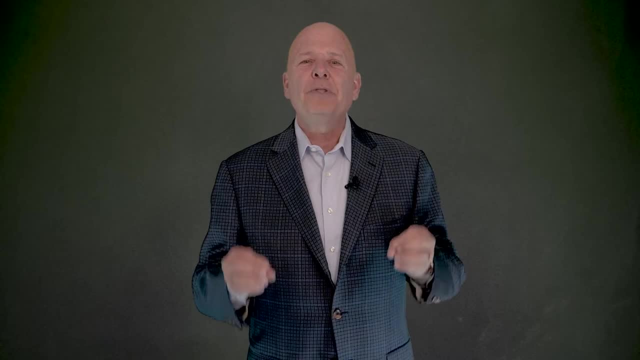 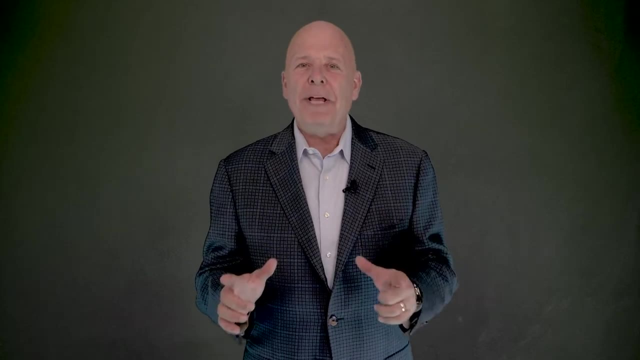 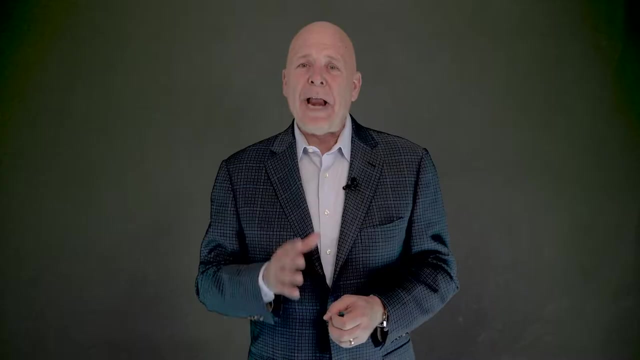 phone. Now that last sentence says it all. Customers call us, but we didn't invent the phone. None of us invented social channels either. His point is just because we didn't invent it And that doesn't mean we shouldn't use it, especially if our customers want us to Now. earlier, I promised to share the why or the reason behind customers turning to social media. While more and more are using social media channels like Twitter and Facebook, it's not always their first choice. Unfortunately, it's where customers go because the company didn't make it easy to call them or didn't respond to their emails or text messages. So they go social and post on Twitter, Facebook and Instagram, And that's the reason why customers turn to social media, And that's a terrible reason. And, by the way, the rest of the world can see these posts And if you choose not to respond, your customers might notice. Yet, despite that terrible reason,